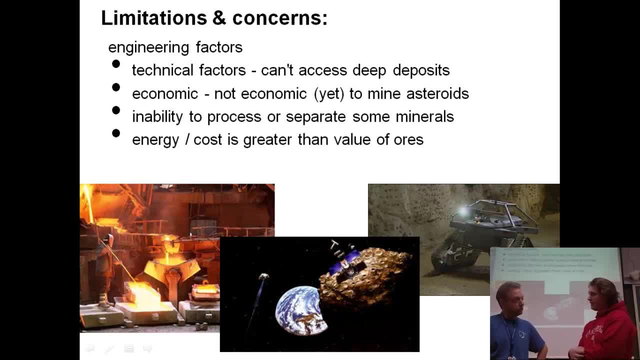 Okay, Inability to process or separate some of the minerals- and this is kind of going back to that ore question, right, Because we talk about some ores mixed in with other rock and we have to separate those and that's where we get that gang or those tailings, right. 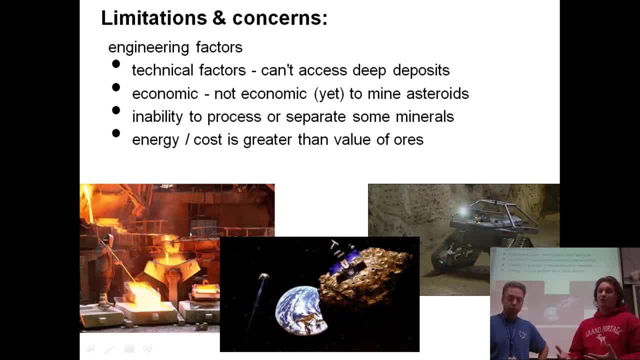 But sometimes it just costs too much money to separate them and it costs more than what the mineral or the ore is actually worth. So then it's really not economically feasible to do that. So maybe like something's stuck with something and it's too difficult, too much money to like separate it, or like oils and shale but to squeeze it out of the shale, they can't figure out how to do that economically yet. 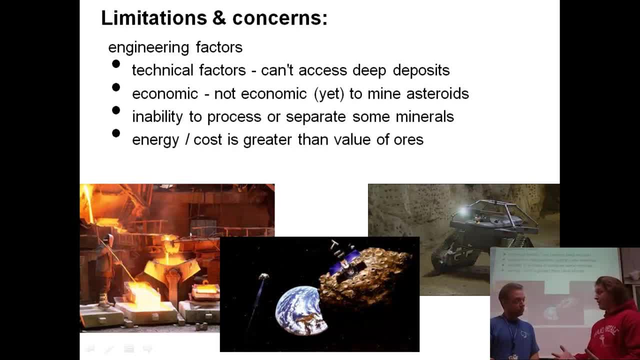 Yeah, they almost have to. they have to spend too much or use too much energy to get the oil out of the shale. so it's: you're taking so much energy to get that oil energy out and it's just like an energy negative. 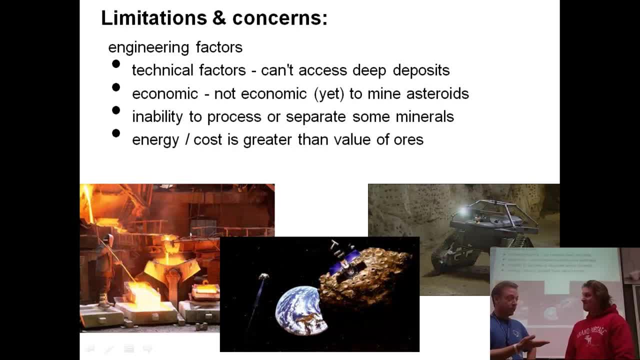 If our kids could figure this out, they could change the world and become the next like billionaires. They could, and I hope they would keep either myself or you or Mr Baldwin and Ms Awad in mind when they do that. Yeah, remember us. 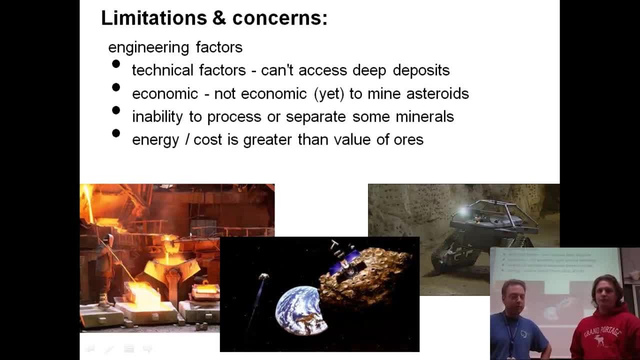 So remember us All right. so then you said energy cost is greater than the value of the ores, and that's what you were just saying. Yeah, and we just kind of talked about that too. It just takes more money to try to get that. 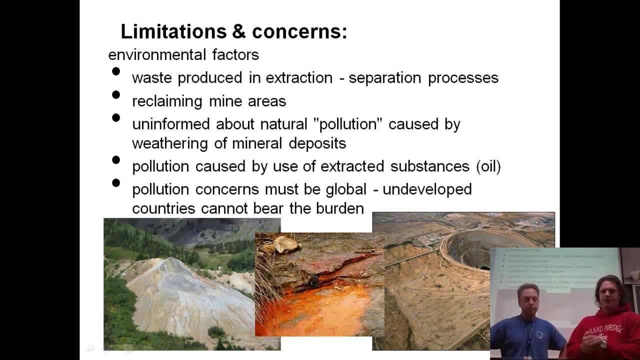 Exactly All right, moving on. All right. limitations and concerns continued. Now we're looking at the environmental factors. That doesn't look very pretty. No, it doesn't. It doesn't, And it was kind of touched upon a little bit in the last segment. 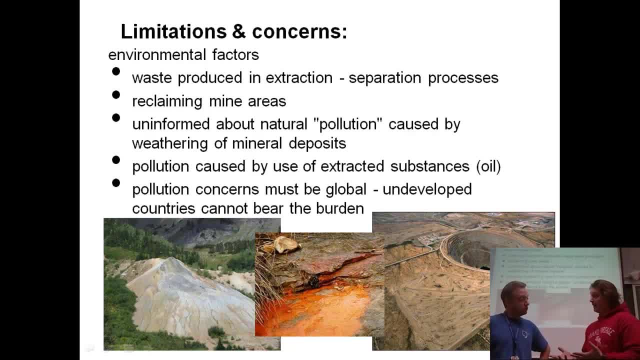 Okay, Especially where we talked about the mountaintop mining and we talked about different things that are destroyed during that process, or the strip mining too as well, where we just kind of strip away the entire earth. So we know that there's going to be other impacts on other people, animals, the environment, et cetera, that we also have to consider. 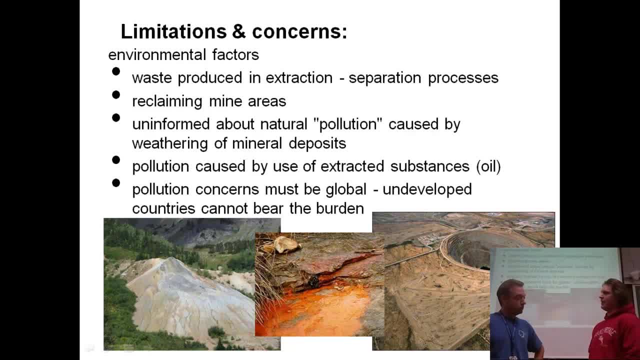 So waste produced in the extraction. so, taking a look at that, What kind of waste is produced? sometimes- Well, you were talking about gang. One of the minerals- that is gang- might be like a hydrogen sulfide or something. So they take a valuable ore out of it and they're like I don't need this rock rich in hydrogen sulfide and they kind of make it a pile. 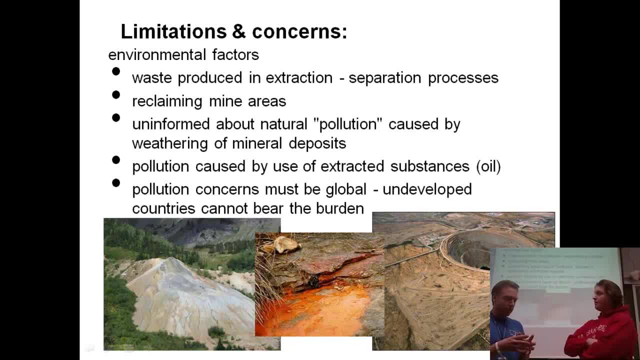 Yeah, And you get acid rain eating it away and then you could get like sulfuric acid or something leaking into the groundwater. that affects the poor people, something like that. Sure, yeah, or it affects people's homes, right? I mean it just leaches into the groundwater and then eventually can contaminate that. 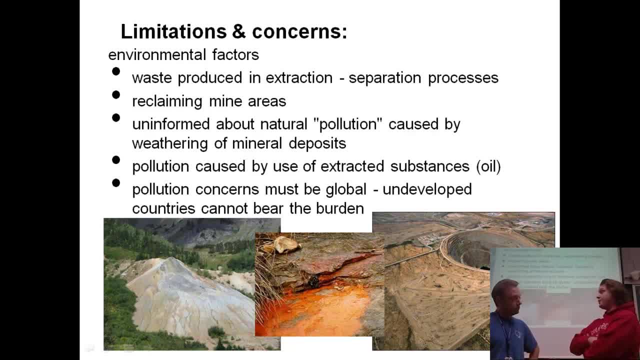 And sometimes these aren't really seen for years. down the road It accumulates over time, Exactly exactly Reclaiming the mine area. Okay, so you can go and you can take the top off of a mountain, but can you feasibly put it back? 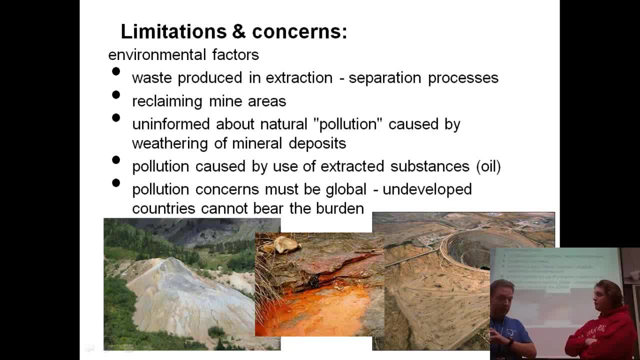 If you're gold mining and you take all the trees, then can you really put the trees back. That's a little easier, but I don't think they can put the top of a mountain back. No, I don't think so either. 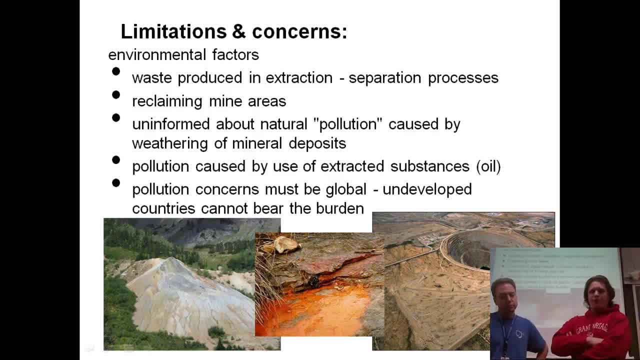 So that's a limitation. Yeah, Uninformed about natural pollution caused by water, Uninformed about pollution caused by weathering of mineral deposits, And that's kind of what we just talked about. right, You know we have these deposits of tailings or gang and you know it rains. 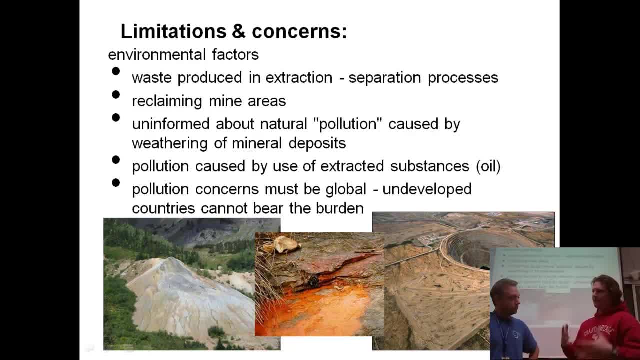 We would get sulfuric acid as just an example, and that would then leach into the groundwater and possibly cause a contamination, But that uninformed. I'm a little confused about that. Well, let's say you're the mayor of Zeesville and I'm a miner and I'm- hey, I want to get some gold from your property. 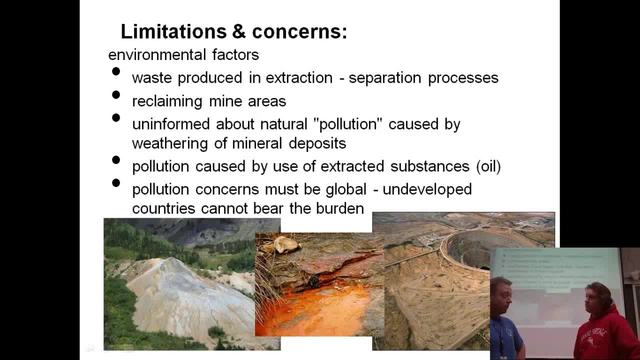 I've got 25% of what I get. That sounds good to me. Oh yeah, I see your town's kind of poor. Okay Yeah, Now you give me. you ask me for an environmental impact survey, So I give it to you and you look at it. 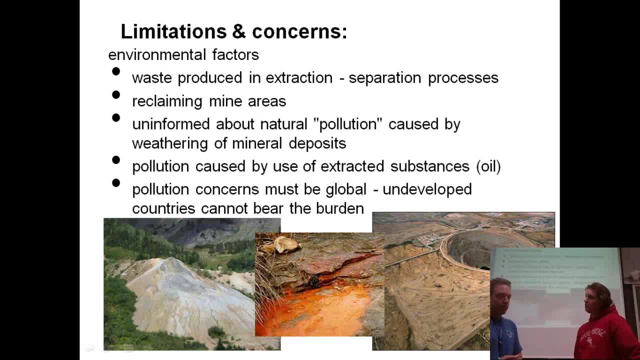 Oh, it's pretty safe for my town. Sure, I neglect to let you know. maybe you know that some of these tailing piles can actually leak And, like you said over time, or maybe I'm not- I haven't started mining and I'm not even informed enough. 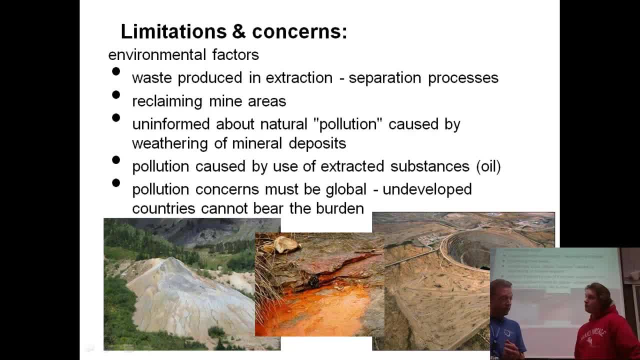 I'm not even sure, and I didn't pay somebody to do studies to find out. So you're getting money, I'm getting money, And then all of a sudden, before we know it, now there's problems neither of us saw. 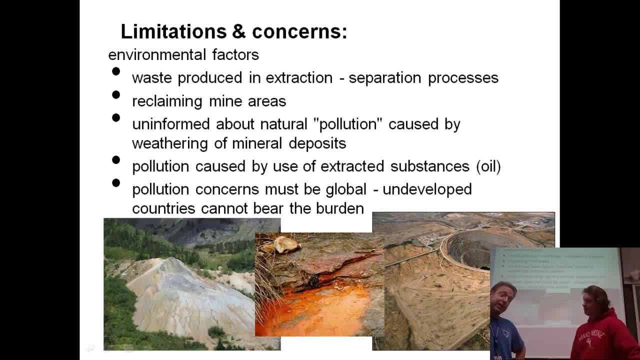 Yeah, and then you're probably long gone by that time. Yeah, that could be. That sometimes happens, unfortunately. Yeah, it does. All right, pollution caused by the use of extraction of the substances. So that's definitely a concern and something that, in this mastery check coming up, that you're definitely probably going to consider. 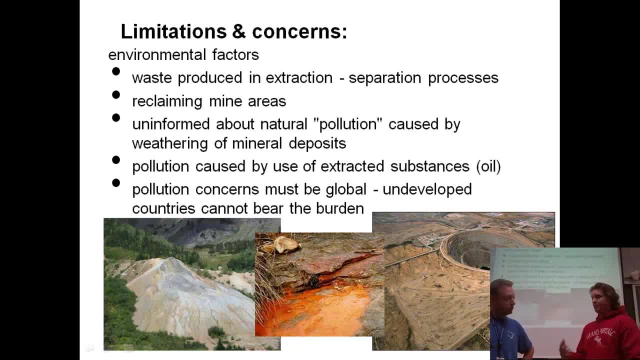 Right, As we actually remove stuff from the ground, there's a lot of machinery and equipment and everything that goes along with it. that is also not- you know, not- good for the environment, So we can talk about that too. Yeah, pump that out of the mine. but if it's not perfect, it can cause pollution. 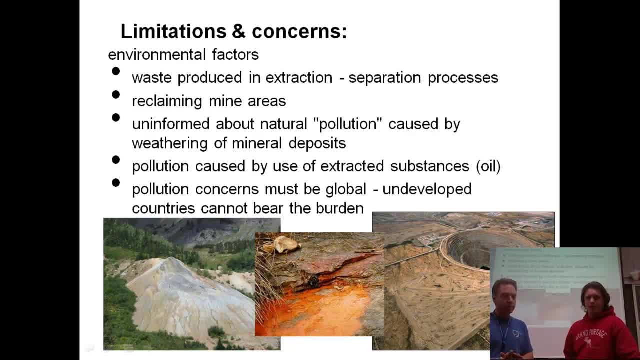 Yeah, definitely. And then pollution concerns must be global. Underdeveloped countries cannot bear the burden. So you mean you can't expect one little country who we're taking all these minerals from to then it's their responsibility then to fix everything. If the rest of the world is like taking their minerals, we can't expect them to like fix it all. 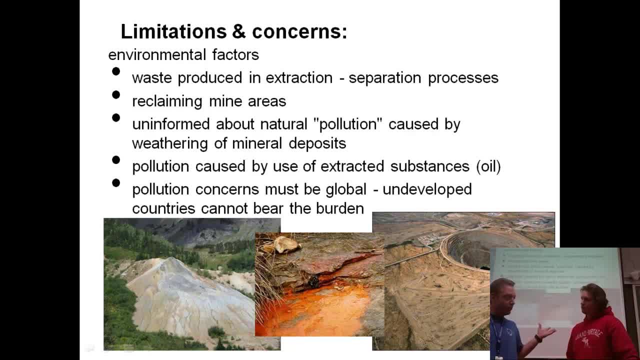 If what they have is going to everybody else, everybody who's getting the minerals and getting the benefits should help them. Yeah, I guess I kind of thought about it a little bit different in terms of a lot of times when they regulate mining, you know. 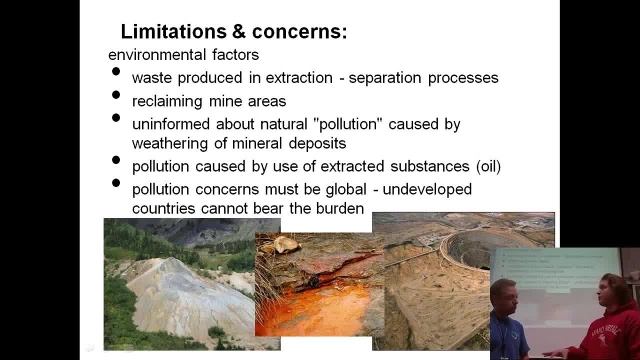 like the United States regulates mining, probably more so than a third world country, And third world countries are just like get it out of the ground and sell it as fast as possible, So they don't follow the same like procedure and protocol that we would in like. 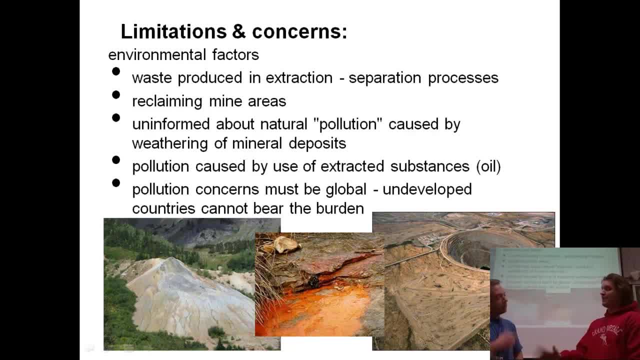 a developed nation- Oh, I see what you're talking about. So a lot of times they can cause more environmental problems, like even in their surrounding area, that they just don't really- I mean, care about, almost. Oh. so, like in that favorite show on mine on Friday nights, they use methods in the jungle gold that they're not allowed to use in the US. 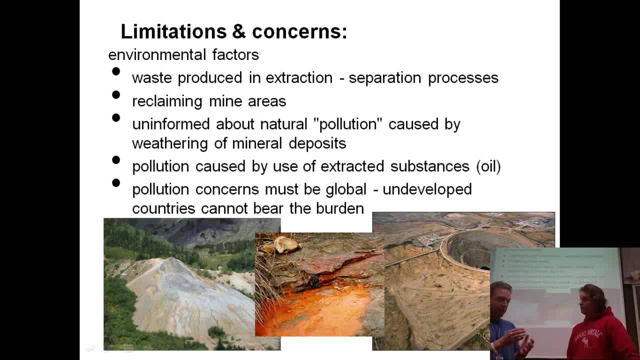 Exactly. So what you're saying- if I'm hearing you- is, if they use the same procedures that keep the environment safe in the US, they should use it everywhere to keep it everywhere safe. Yeah, That's what I'm saying. 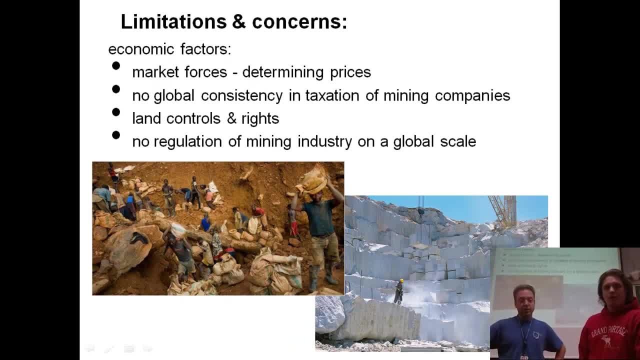 Okay, I understand Exactly All right. So the economic factors that we've already kind of touched upon And going back to, I guess we'll start with the first one here, the market forces determining prices. This is a really interesting one. 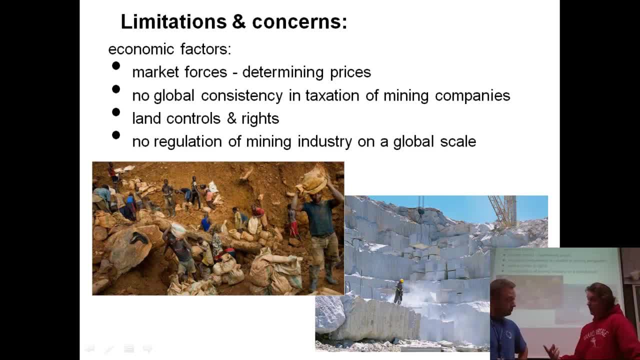 So in our TV show that you and I both watch, Gold Rush- actually a lot of those miners were trying to mine gold in the 80s, Right, But the price for gold was so much lower than what it is today that they actually had to pull so much more gold out of the ground. 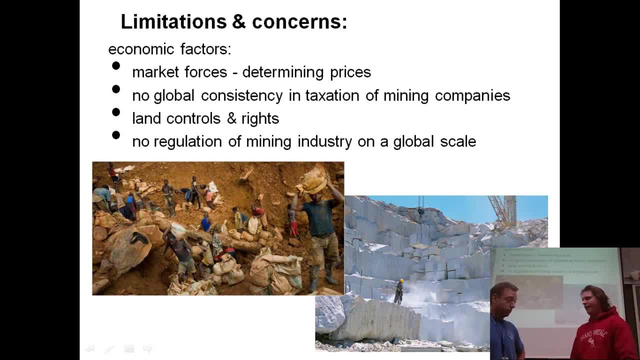 And if there really wasn't that much gold there, they just wouldn't even try. But gold now has, like it's, 20,, 50 times more than what it was back then, Exactly So there's almost like a mini Gold Rush going on back in Alaska because it's just worth so much than what it was before. 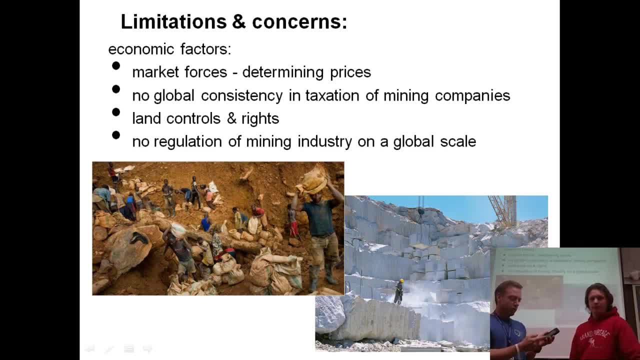 Could it be devices like this too, that there's certain minerals we use in our smartphones and our other devices, that before we never had a need for them and all of a sudden, now we've got a huge desire to have these. Yeah, yeah, exactly. 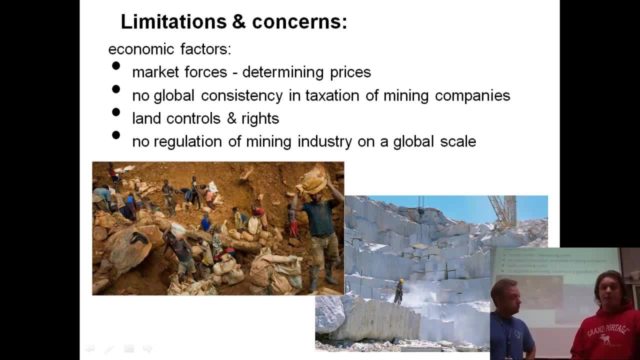 And because the demand is so high, then the price for it is going to increase as well. Okay, And no global consistency in taxation of mining companies. That sounds like what you were saying, where maybe in another country they don't have to pay a certain tax. 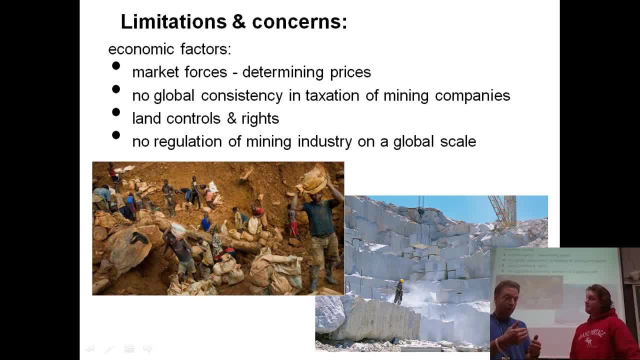 that might go to help reclaim the area, where in the United States they may have that tax worked in automatically on the front end to make sure that things are restored. Yeah, So there should be maybe a global tax that every miner has to pay, and that tax then would be used for reclaiming the area. 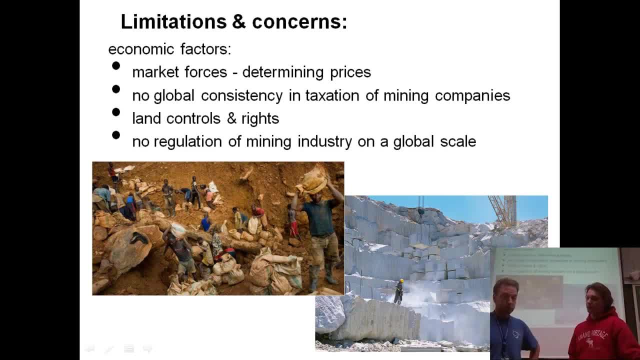 Yeah. or for any kind of research or something like that to Or increasing the yields. Yeah. Land controls and rights. So in other countries, maybe the person who controls the land and their rights might not be the same, And in the US, aren't there even some places where 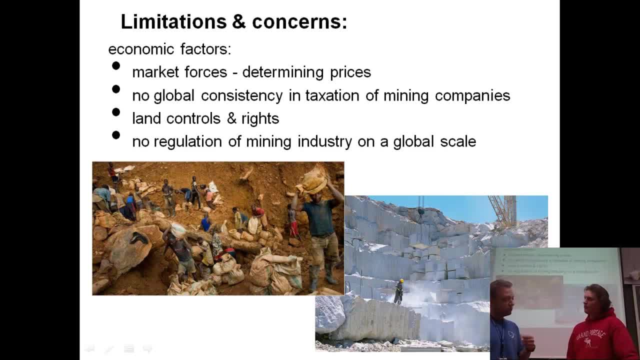 Sometimes you own what's under the ground and sometimes you don't. Yeah, I think so. I'm not actually sure about that. Yeah, I think there's controversy about that. So maybe if we had that standard where it's the same everywhere, 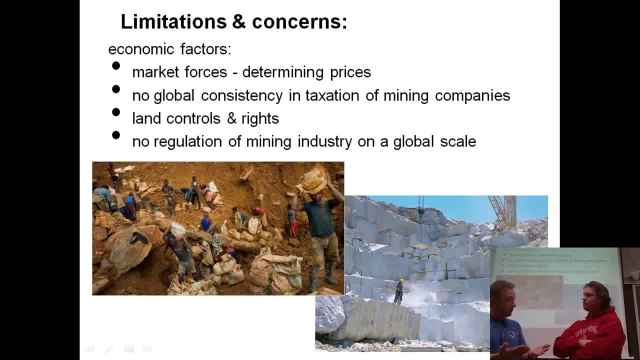 then we could make regulations to make things better and safer and that would help. Yeah, All right, And then no regulation of mining industry on a global scale, And that just kind of goes back to what we've been talking about with a lot of these. 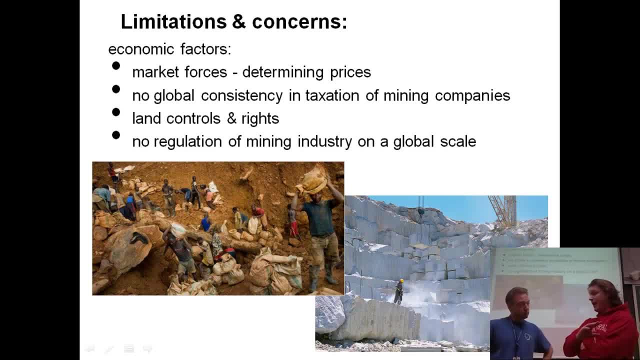 With a lot of third world countries is that just they'll mine it for as long as they can to get all of it out and then move on to a different area. And sometimes that can be problematic for the market too and the economy, if people are producing a lot more of it and maybe in an unsafe way. 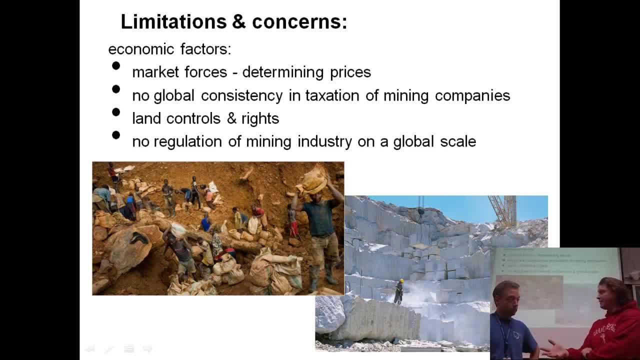 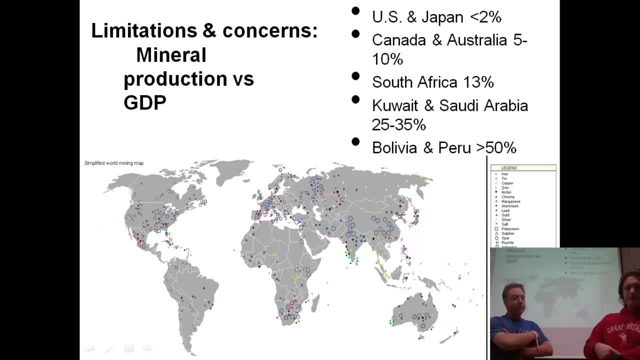 And then other countries may not be able to compete in that same market with the regulations we would have here. So we don't have really a standard regulation globally. that we've actually already mentioned. Okay, That makes sense. All right, We've got limitations and concerns. mineral production versus GDP. 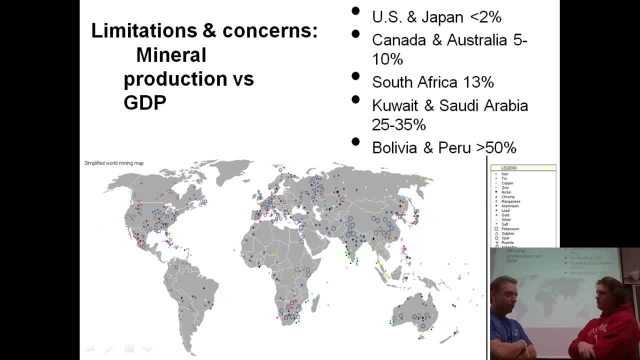 Now GDP, that's kind of like how much a country, that's their money coming into them? Yeah, Okay. So certain countries get more money from minerals than other countries, Exactly Okay. So the US, which is really big, we only get what? 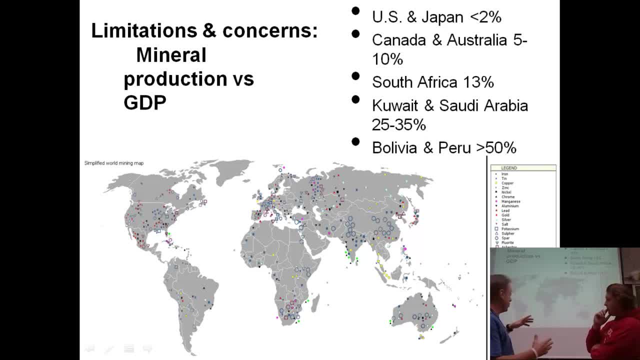 Less than 2% of our. Yeah, I understand Japan, because they're small. We must have other ways that we make money besides minerals, Exactly. And then if we take a look at Kuwait and Saudi Arabia, they're pretty high: 25% to 50%. 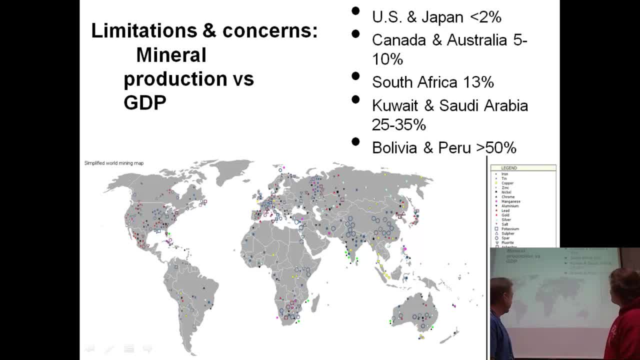 Bolivia and Peru are above 50%. Okay, So if there was some kind of a- let's say a- how do I want to put that- Like a regulatory effect, some type of restriction or control, Yeah, Or anything that would change that market for that mineral that they're mining for, or anything, 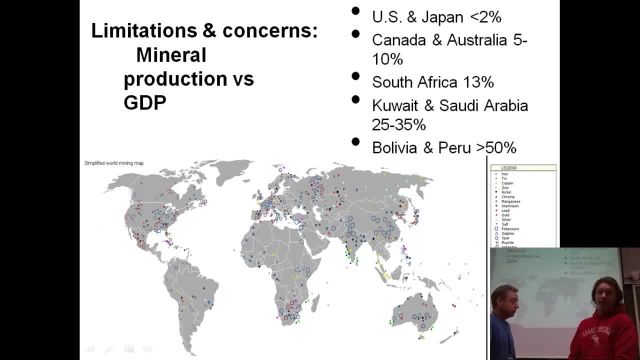 Right, And then that would really have a dramatic effect on their economy, because that's a huge portion of the money that they actually make in those countries. So if we tried to fix this, we might have to try to have a global group that looks at 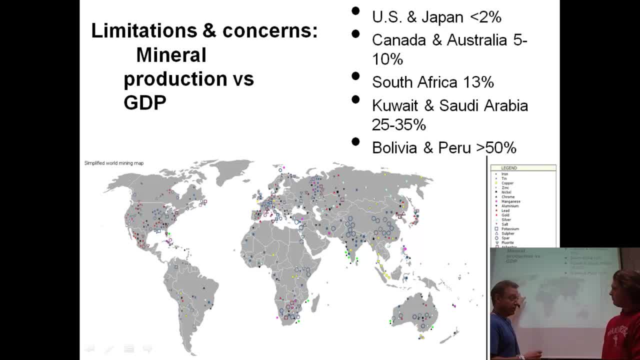 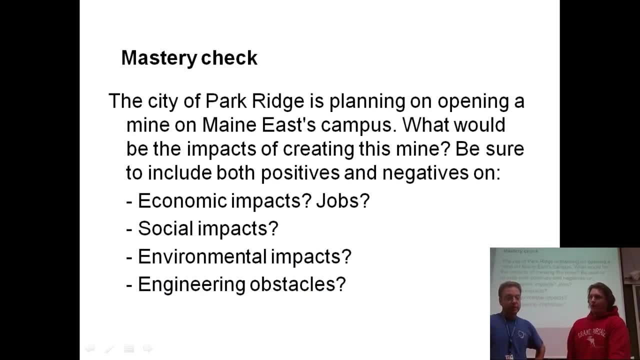 it instead of one major group that looks at it to determine what that would be to make it fair for everyone. Yeah, Yeah, Exactly, Okay, All right, The mastery check. I like this one, Mr Z. Yeah, I like this one too. 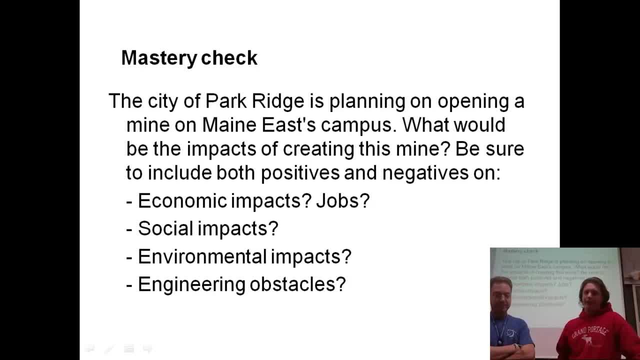 So if you could imagine, The city of Park Ridge is planning on opening a mine on Main East Campus, I wonder what they would mine for. Maybe there's gold there Could be, I don't know. I don't know What would be the impacts of creating this mine. 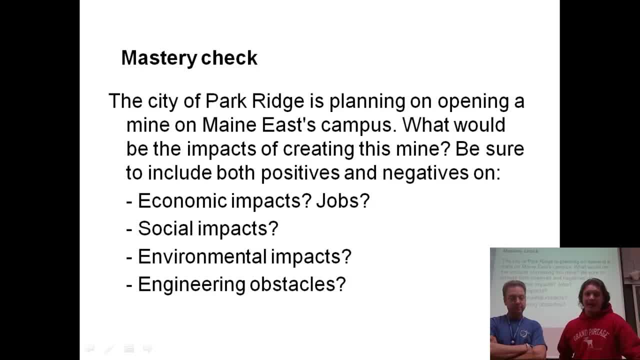 Be sure to include both positives and negatives: economic impacts, jobs, social impacts, environmental impacts and engineering obstacles. So the students should try to think based on what they've seen. If all of a sudden we could mine right here on campus.